is sales tax. In general, paying sales tax means it's retail. Wholesale usually does not charge sales tax. This is because in most states you're exempt from paying sales tax on items that are going to be resold with the proper permits and documentation. But it's not just a discount. 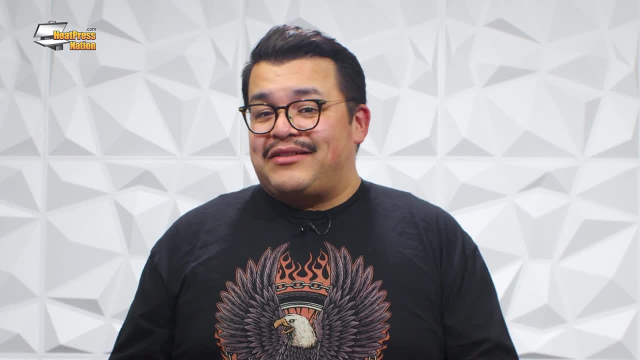 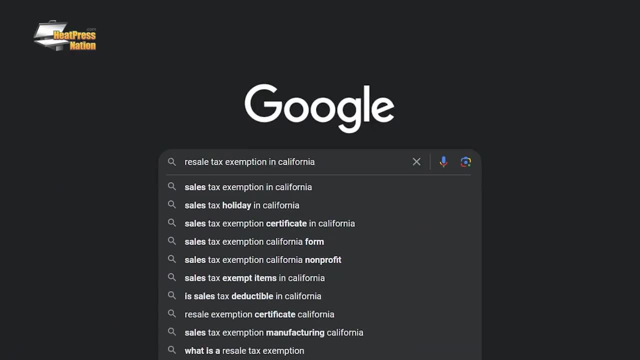 You're also required by law to collect and remit sales tax when you eventually sell your finished products. For more information, just google resale tax exemption in your state and that should give you the link to the proper government entity in your state. Now it does vary. 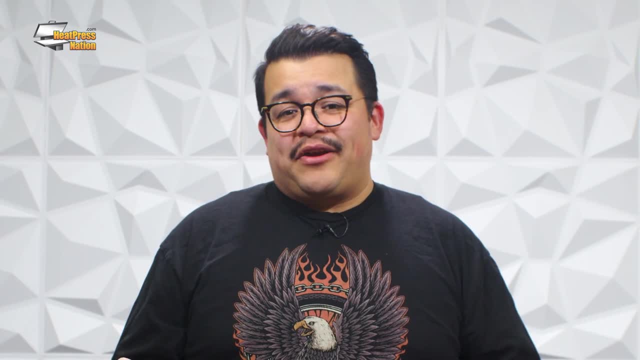 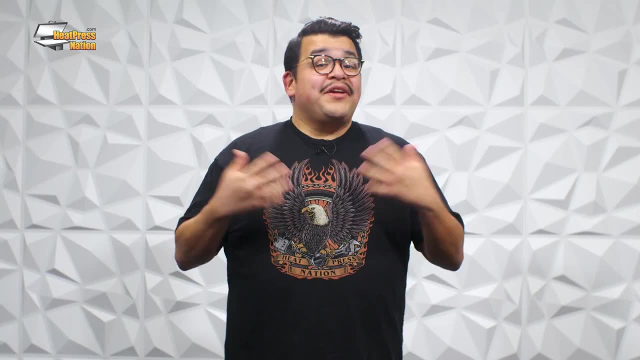 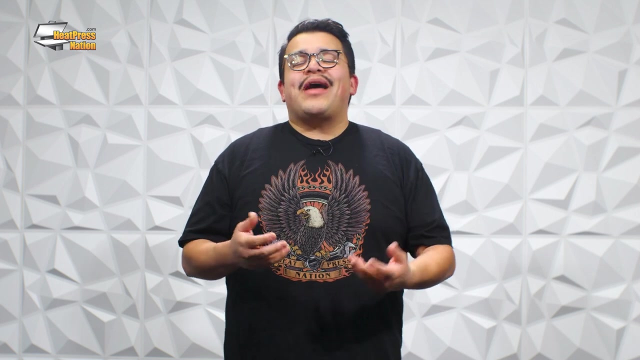 state to state, so I'm not going to get into specifics in this video. I will say that where I live, the average sales tax rate is between 8 and 10 percent- California. So if I'm ordering $200 worth of blank t-shirts, I can save $16 to $20 on sales tax just by having my reseller's permit. 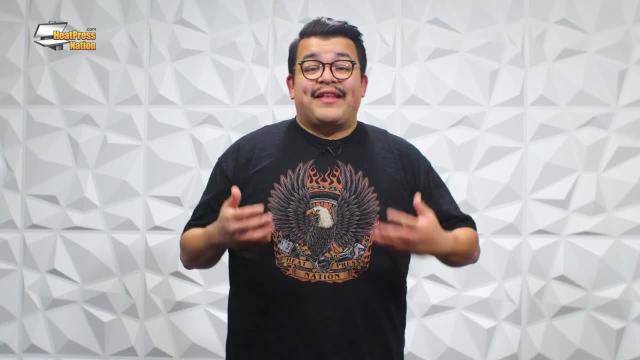 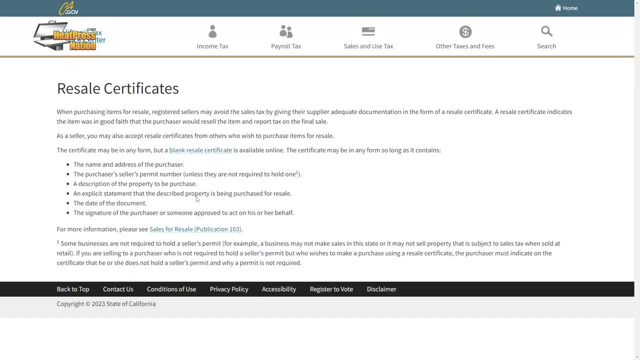 in the state of California, And that's on top of the lower price that I'm getting from my wholesale supplier. So here's my advice to you on sourcing your materials: Find out what it takes in your state to get your tax exemption for resellers and follow through with it. Then find at least two. 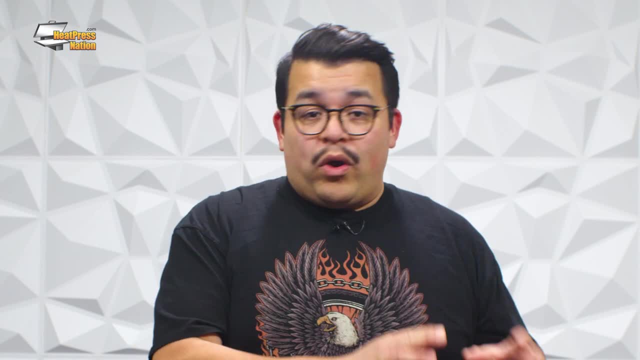 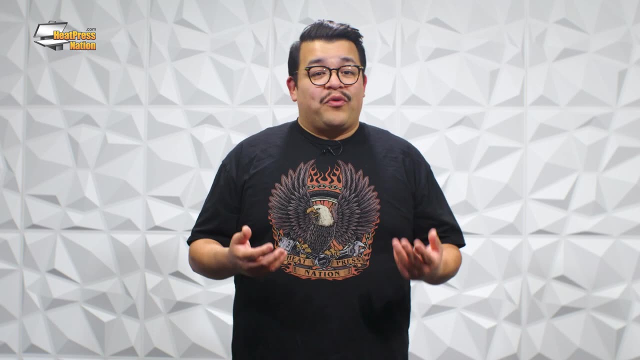 or three wholesalers and open accounts with them. Sometimes one place may run out of your favorite t-shirt, so you'll need access to another source. Some popular brands also sell wholesale direct, but only if you have your sales tax exemption in your state. Different suppliers have different. 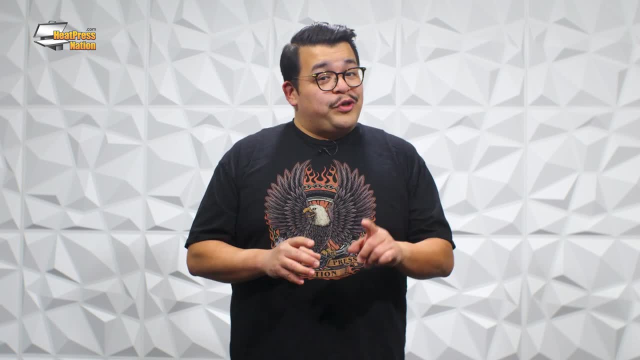 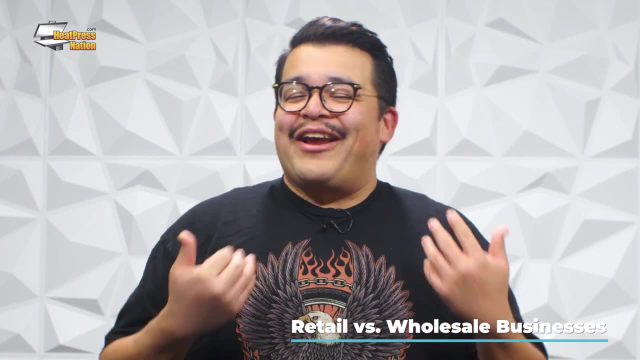 minimums. You'll see inside the description below that there are going to be different rates, shipping costs and turn times, so be sure to do your research before ordering. Now let's talk about retail vs wholesale. for your business In our industry, here's an easy way to know what's what. 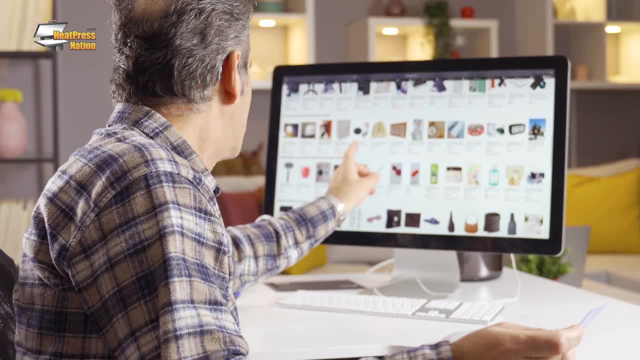 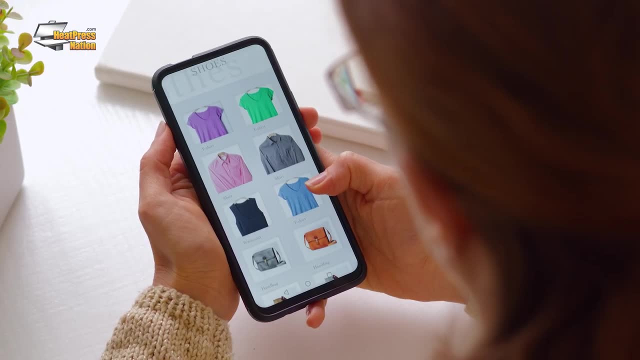 Retail products are purchased by the end user. If you have your own company, brand or clothing line and you sell direct to consumer or DTC, you are, in fact, a retailer. Now, if you make custom orders for your clients, that is also an example of a retailer. If you are selling products from your own company, whether you are a customer or a retailer, you are a retailer. 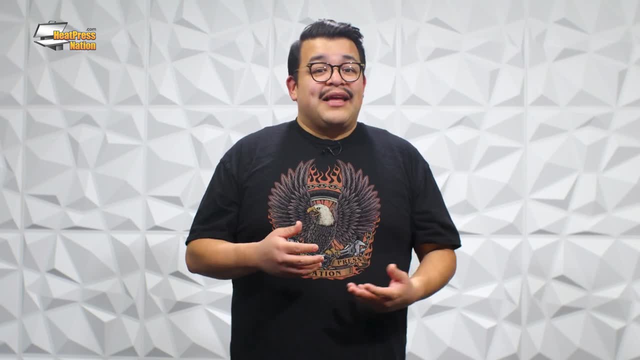 If you have a website, you are a retailer. If you are a customer or a group, you are a retailer. If you have a seller, you are a retailer. If you are a customer, you are a retailer. If you make custom orders for your clients, that is also considered retail. 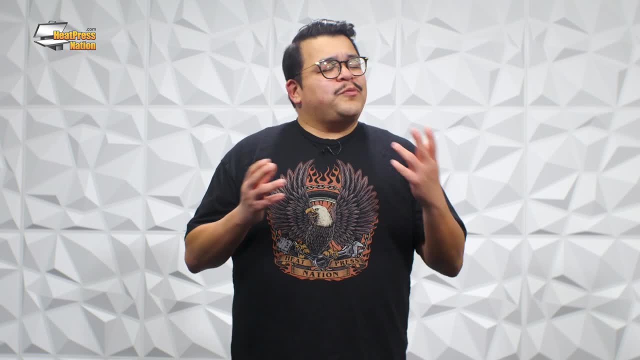 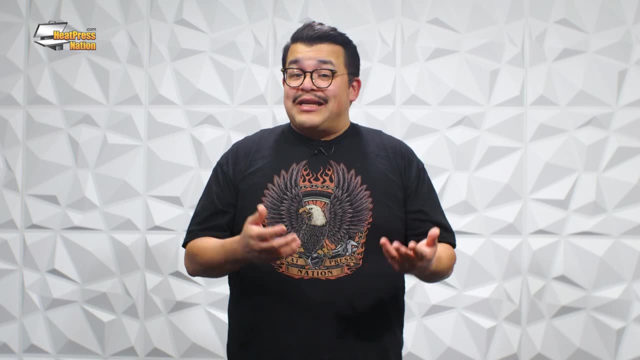 There are different ways of selling DTC, but in our industry, the most popular methods are going to be through Etsy, your own website, in person at pop-up shops or events, and sometimes even through DMs on social media. A big advantage to selling retail is going to be your profit margin. Because you're the maker and the seller. there's no middleman marking up your prices or cutting in on your margin. Your customers get the best price possible and you make the most money per item sold. The downside is that you're responsible for all of your own production, fulfillment, marketing. and customer service. so you are going to have to work for that extra margin. Wholesale products are purchased with the intention of being resold, usually in bulk. If you are taking large quantity jobs, if your customers sell your products to their customers, or if you have a brand or clothing line and sell to stores, Of course there are exceptions to what I just said, but these are generalities. A lot of the work in wholesale is going to be sales. Instead of selling your products to people or individuals, you have to sell to stores. If you're just getting started as an independent maker, it's probably best to start by targeting. 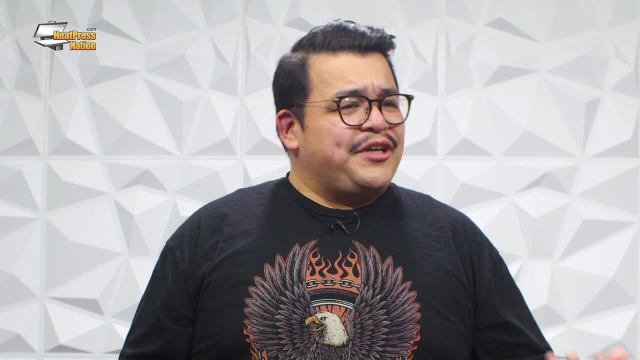 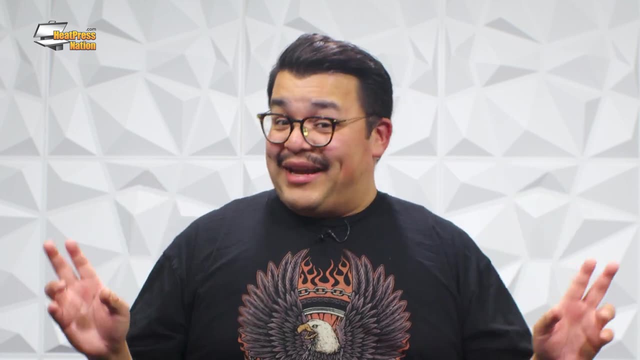 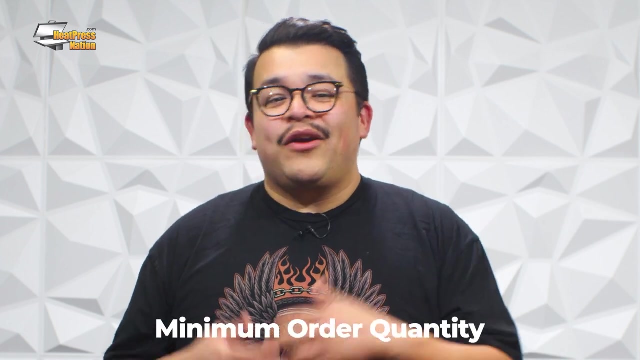 independent shops, Boutiques, skate shops, sneaker shops and gift shops are great places to start. You'll be selling at a lower price per piece than retail, but the benefit is that you're selling more items in one shot thanks to something called Minimum Order Quantity or MOQ. 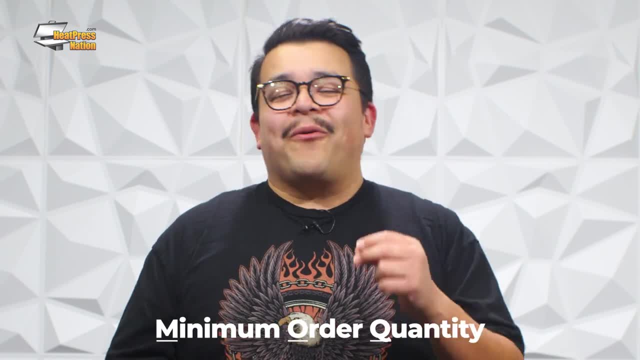 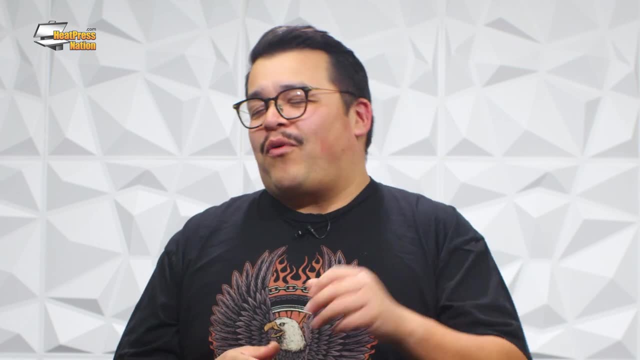 This is the minimum amount of items a store needs to purchase in order to get a discount. There's way more to talk about that's not going to fit in this video, but here's a quick example of what I mean. Let's say you have an MOQ of 10 at $14 per tee. 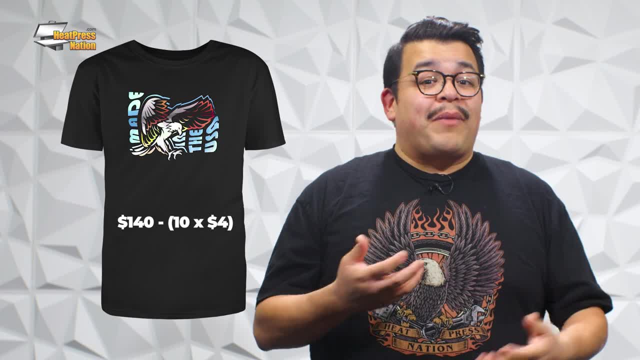 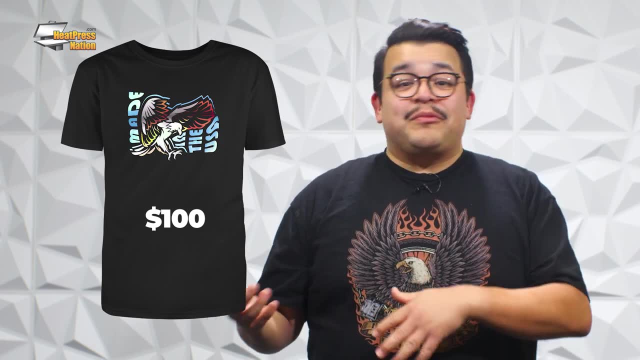 That's a $140 order in one shot. Each shirt might only cost $4 in materials, so you just made $100 in one order. That's it. You don't have to ship 10 different orders to 10 different people and get 10 different. 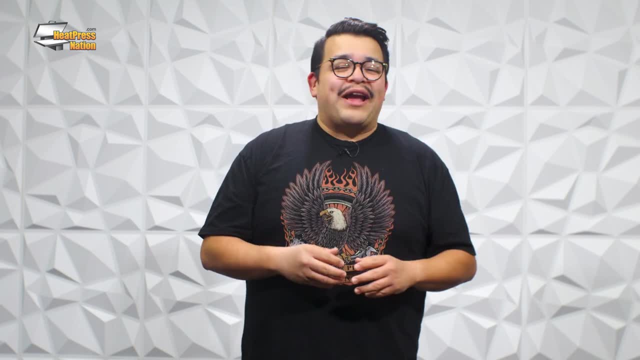 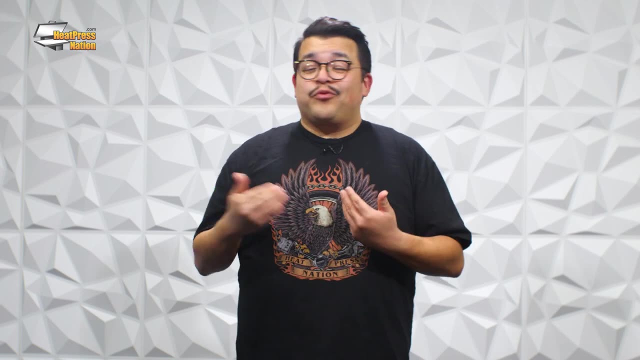 inquiries of when's my order going to arrive. As your brand grows and develops the following: it'll be a lot easier to get your line sold in even more stores and possibly even chains and major retailers. As your orders get bigger, the cost per piece will go down, but your overall revenue will. go up. When wholesaling, you have to consider that many larger businesses operate on net terms. This means you may not get paid until 30,, 60, or even 90 days after fulfilling your orders. Whether or not you want to accept net terms is up to you, but you will definitely want. 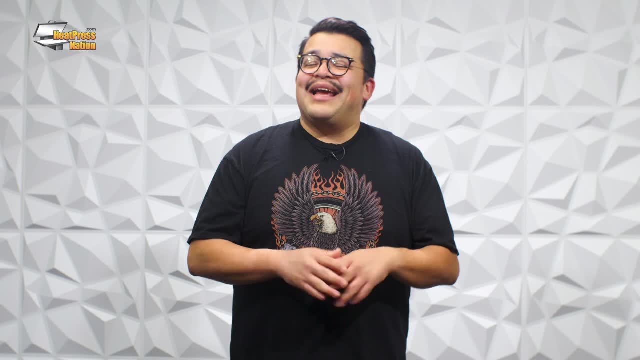 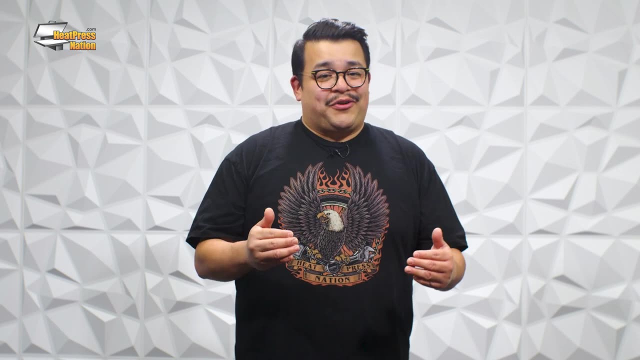 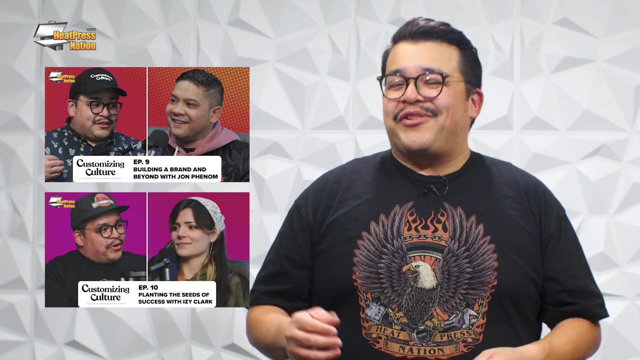 to do your research on invoicing and purchase orders. I cannot talk about wholesaling as an independent creator without mentioning two specific episodes of Customizing Culture, The Heat Press Nation podcast. Go listen to episodes 9 and 10 with John Phenom and Izzy Clark respectively. 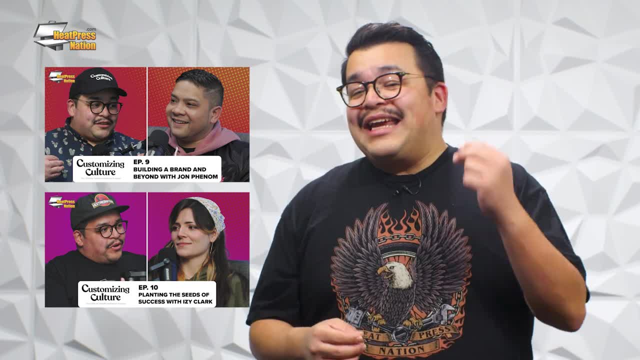 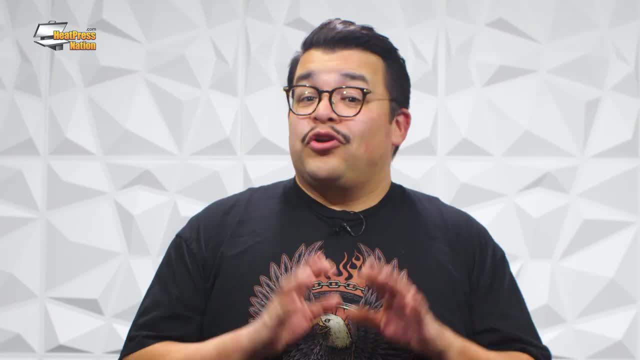 They share their stories and bring some great, fantastic insider information on selling wholesale as an independent creator. The links to each episode are in the description below. Trust me, this could very well be the inspiration you've been needing to start wholesaling your products. 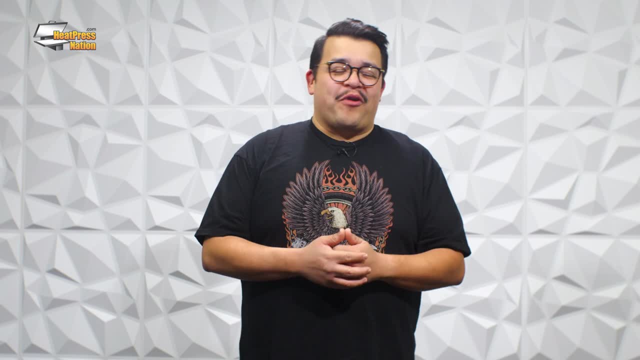 We'd love to hear about what method you prefer for selling your products. Let us know in the comments below or over on our website. We'd love to hear from you. Don't forget to subscribe to our YouTube channel or over on our Facebook group: Heat. 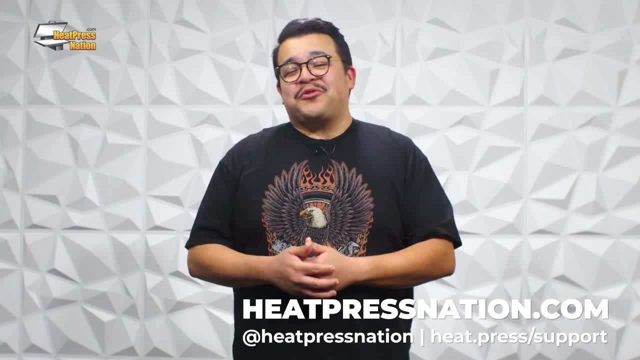 Press Nation Creators. For more Heat Press content, be sure to subscribe here on YouTube. And don't forget, you can get all of your heat transfer supplies over at HeatPressNationcom.